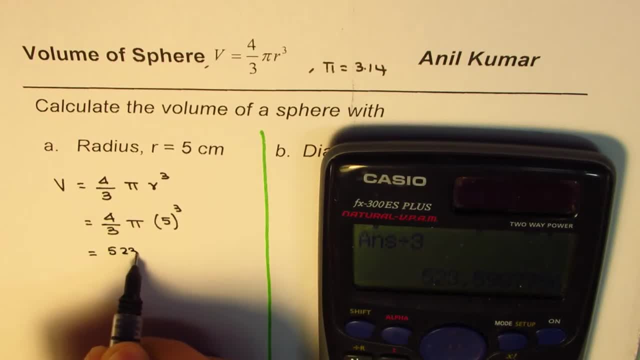 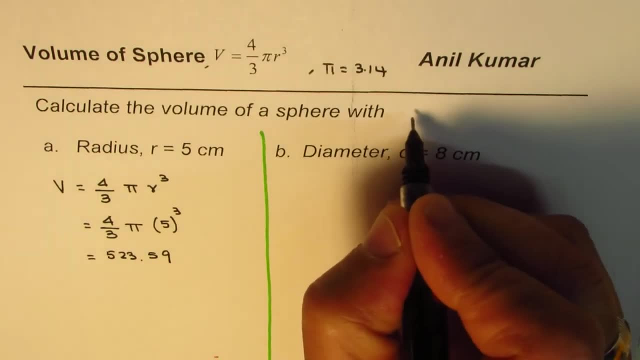 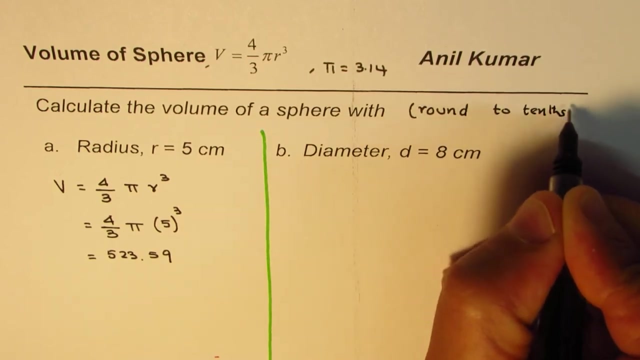 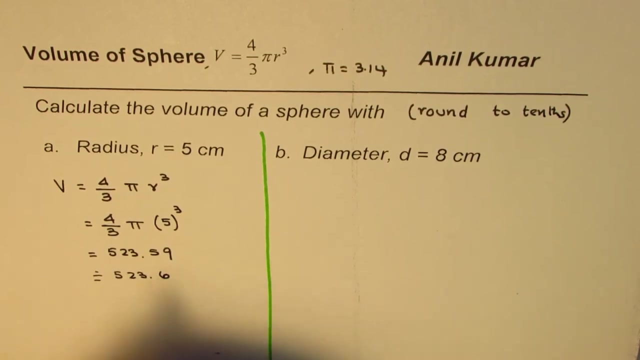 equal to 523.59.. So let's round this answer to one decimal place. So okay, so we'll round the answers to- let me write down here- round to tenths. So if you round to tenths one decimal place, you get this as 523.6.. And what should be the units? 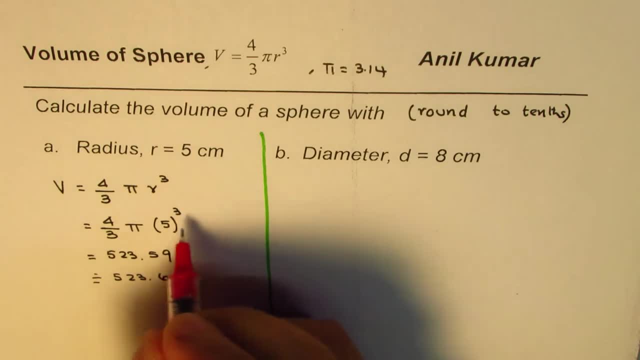 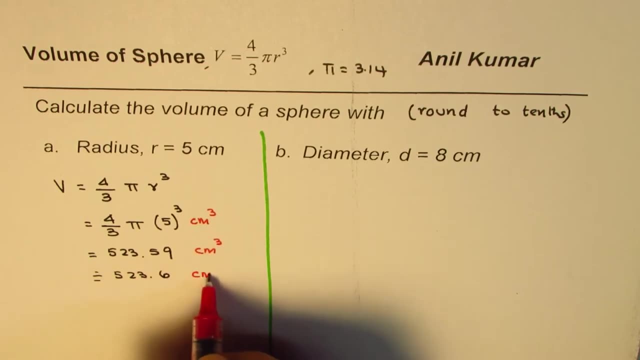 Well, let's look into the units. r is in centimeters, So this becomes centimeter cube. Is that okay? So the units will be centimeter cube, So we can write down our answer. That is the volume: v equals to 5.. 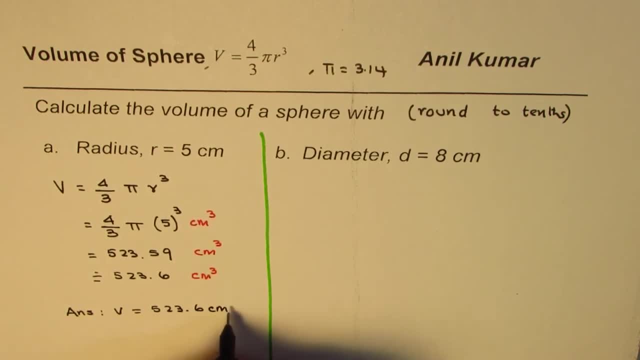 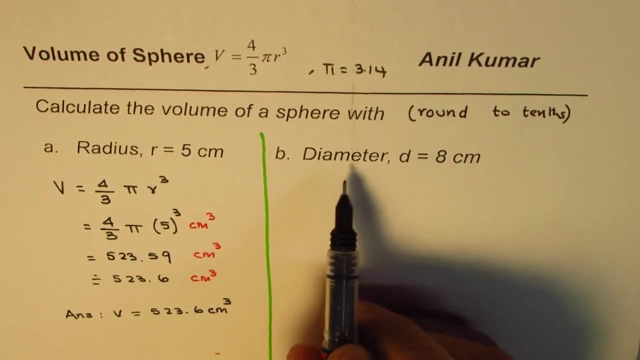 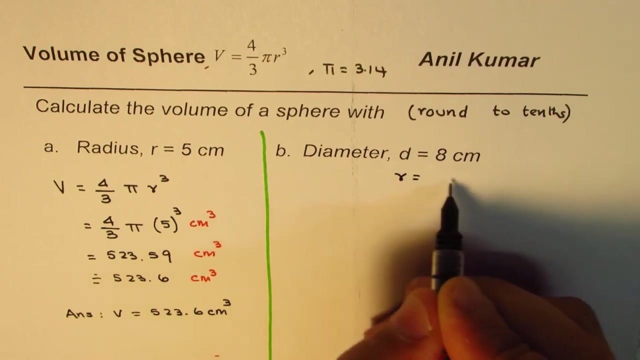 23.6 centimeter cube. Alright, So let's do this exercise once again for the second example. Here we are given diameter t equals to 8 centimeters. Now if diameter is 8 centimeters, radius should be half of diameter right Diameter divided by 2. that 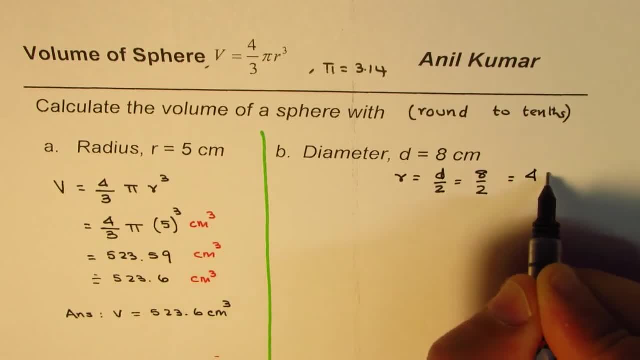 is 8 divided by 2, which is 4 centimeters. right Now we have to apply the same formula: volume agreed to zero. That is when what that unity Yea is equal to 3 times pi by 5.. Remember, f of 5 is 5.. So let's do itzin to 7 times pi of gain, Every second is equal to 0. So if we give 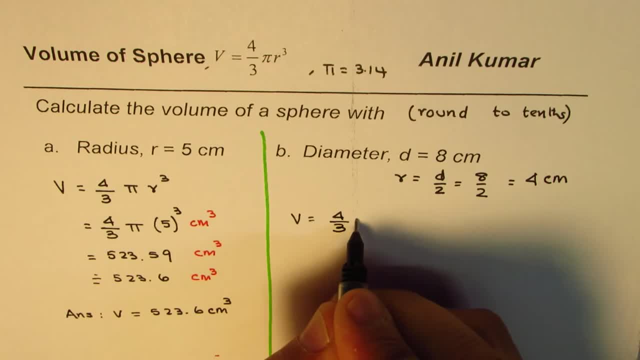 us an appleлуш. so this equals to 4.5 times pi by pi. Now, if we divide this all by, equals to 4 over 3 pi r cube, which is 4, right, so you could also write this as 4 centimeter. 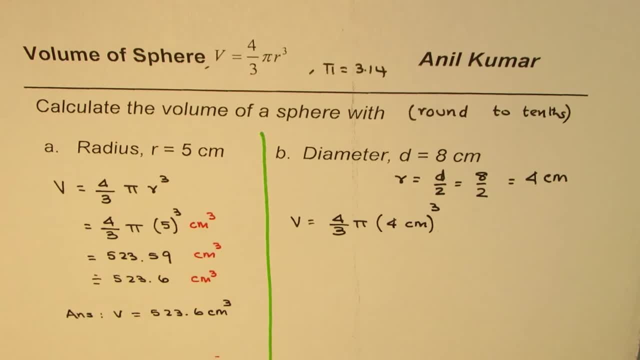 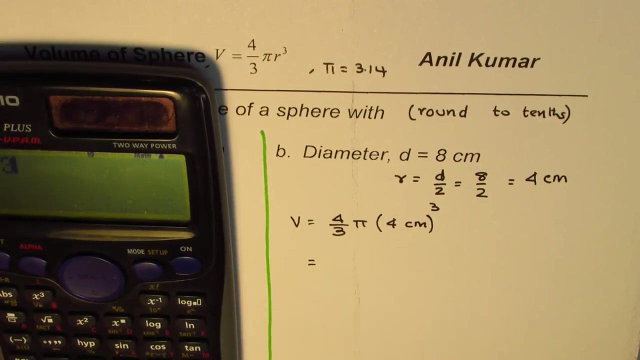 whole cube, is it? okay? so that is how you write and then you can calculate using the calculator. okay, so this time what we will do is we will first divide. so what we can also do is we can do: 4 divided by 3 equals to. then we'll do times pi. so instead of writing pi, i'm writing 3.14 this time. 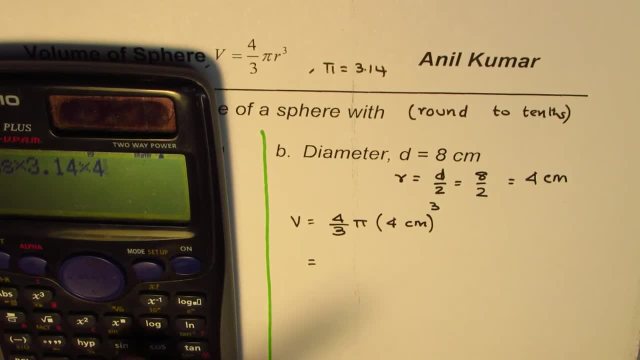 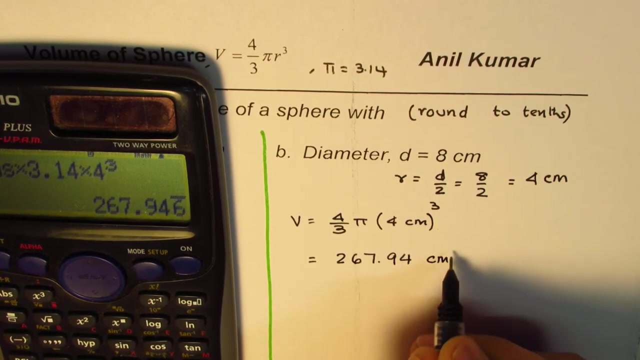 right times 4 cube. times 4 cube equals to: we get some answer in decimals. this gives you 267.94 right centimeter cube. rounding this to one-tenth will give us, because this 4 is less than 5, 267.9 centimeter cube. i hope the steps. 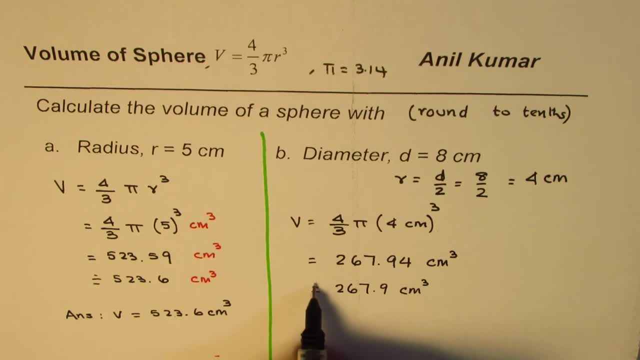 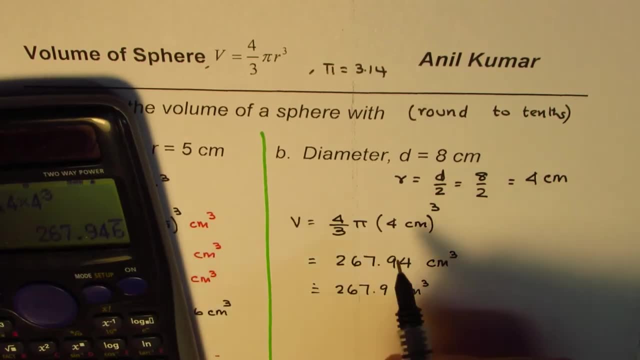 are clear, right? so that is approximate, since we took an approximate value of pi 3.14. well, this was with. let me write down here: this is with: pi equals to 3.14. so Now, if I use pi not as 3.14, but as pi, let us check the value of that also, right? 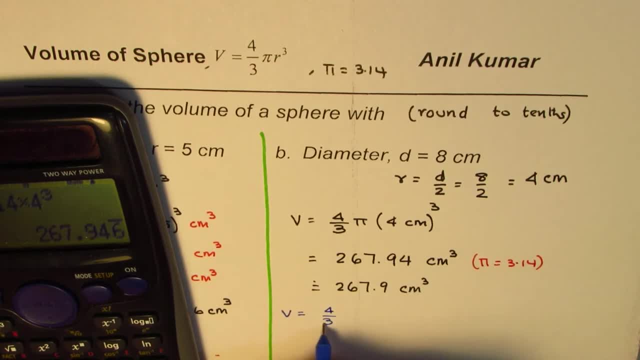 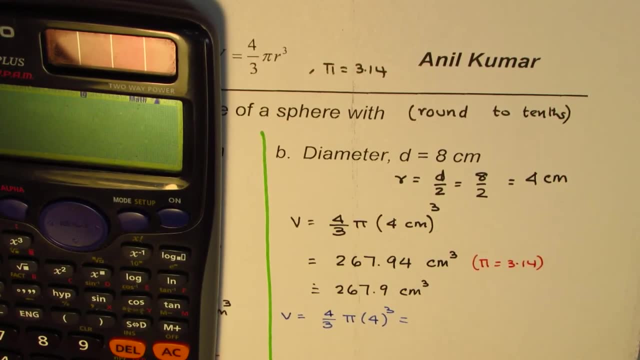 So we will do again the same calculations: 4 by 3, we will use pi, this time 4 cube. okay, let us do it. So we have 4 times pi times 4 cube, right? So this gives you that answer, divided by 3 equals to: in decimals, we get 268.08,. do you see that? 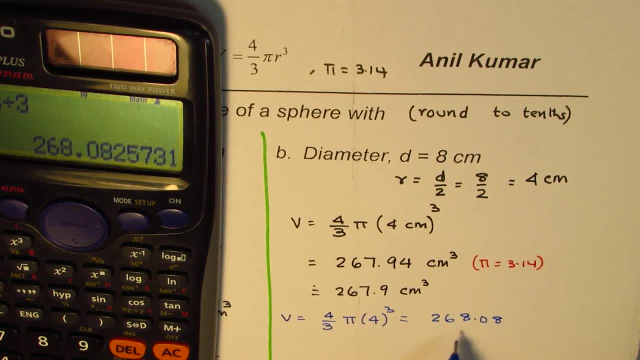 So we get slightly higher value, right? So this could be approximated to 268.1 centimeter cube, right? So that is the difference. and the difference is mainly because when you use the value of pi and when you say what is this equal to, I mean sorry. 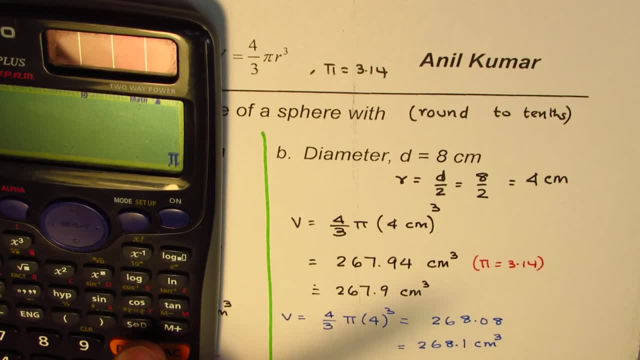 if you use the value of pi equals to in decimals, it is actually so, because pi is actually equals to 3.14159- something, something right. So we use 3.14 in our calculations, which is roundabout correct value. 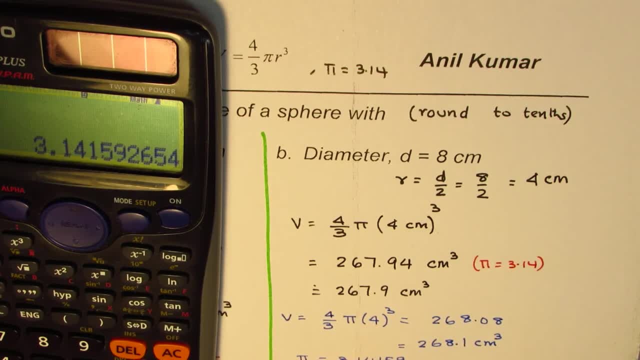 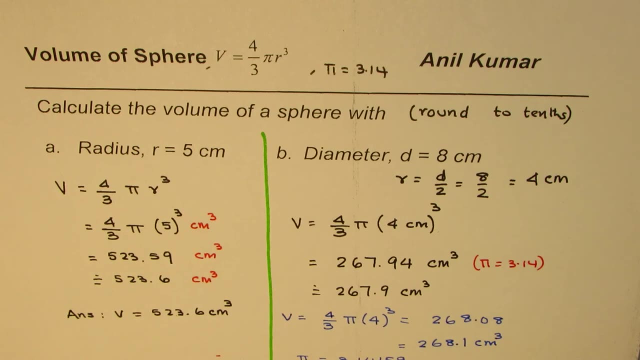 but 0.04.. So this 3.14159 makes slight difference when you multiply some big number and you can get difference to 1, 1's place correct, as you can see in this particular case. So there could be some error by using 3.14, but that is kind of acceptable. 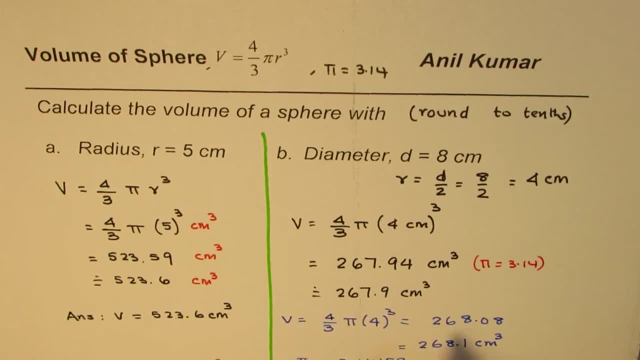 if you are rounding them to 1's place. So if I round to 1's place here, I could get this approximately as 268.. 268 centimeter cube and here also we get 268 centimeter cube, right, sorry, cube. surrounding to the one space, 3.14 is good enough to use. that's what i want to. 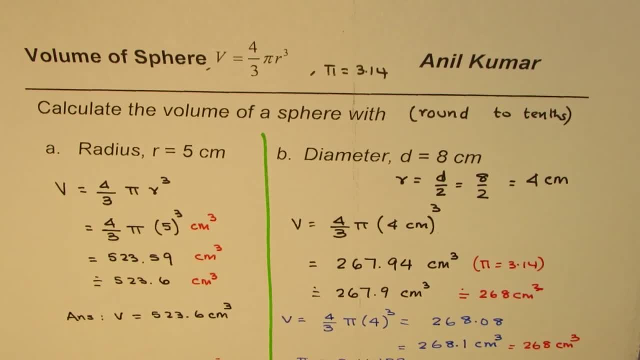 suggest at this point: right? i hope that helps. thank you and all the best.